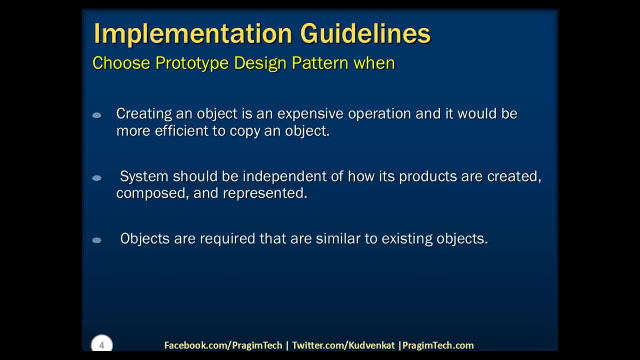 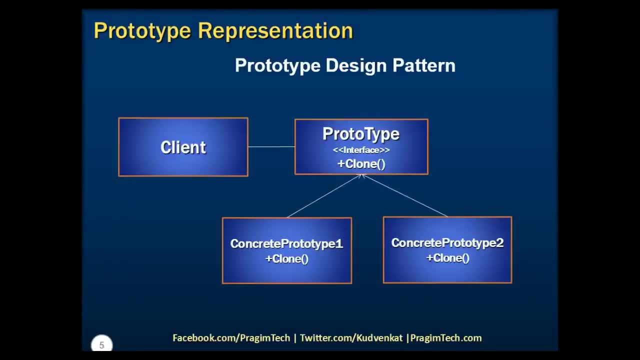 are required that are similar to existing objects And when we need to hide the complexity of creating new instance from the client. Now, if you take a look at the illustrated diagram of prototype design pattern representation: client represented here- creates a new object by asking a prototype to clone itself. Prototype- 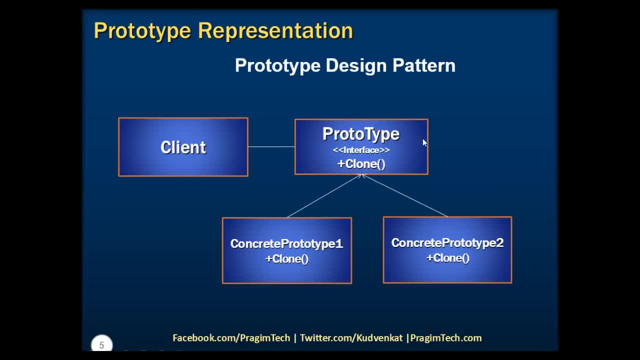 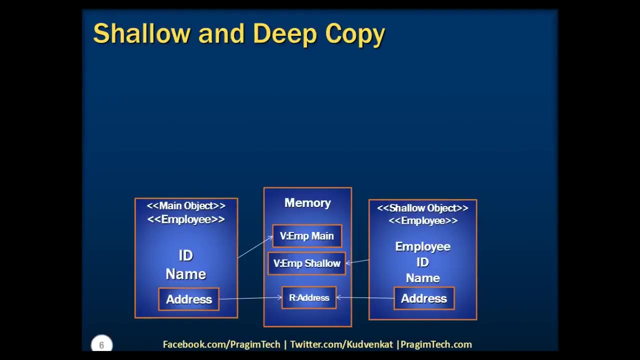 specifies an abstract interface for cloning the required object And concrete prototype implements the prototype interface for cloning itself. Let's now understand the significance of shallow and deep copy in prototype design pattern. The idea of using copy is to create a new object of the same type without knowing the 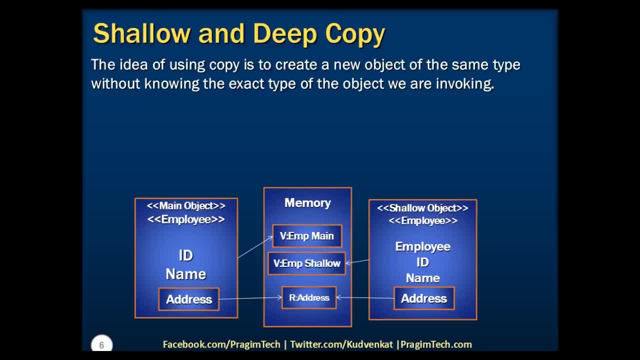 exact type of the object we are invoking. Shallow and deep copy are the two mechanisms used in copying an object. Let's now understand each of them in details. If you take a look at the representation diagram of shallow copy, the main object here consists: 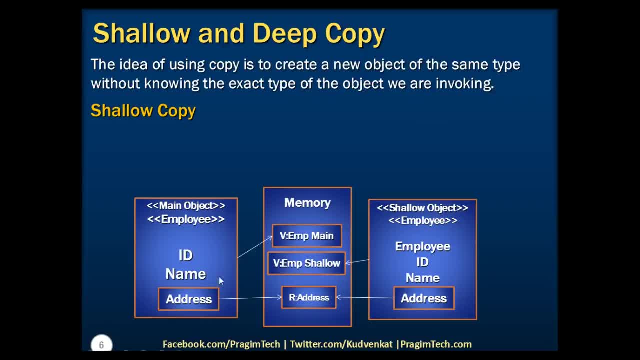 of employee details such as id name and address. Once we perform the shallow copy of the employee object, You may notice that both the main employee address object and the copied employee address object are referring to the same address location in the memory, Which means shallow copy copies an object's value type fields into the target object and 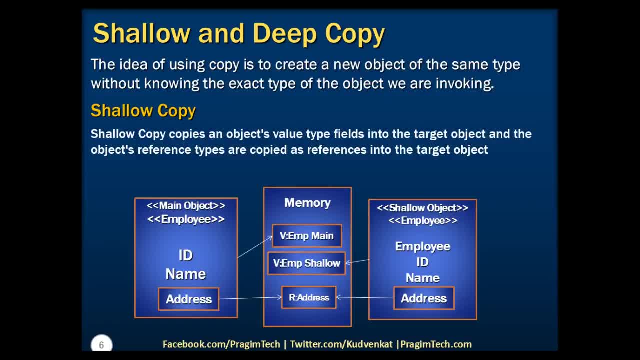 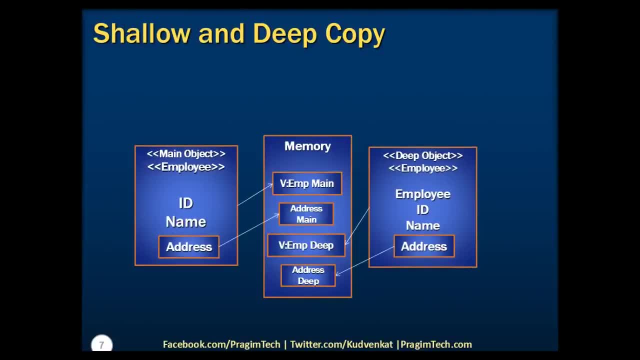 the object reference types are copied as references into the target object. I hope now you got an idea of shallow copy. Let's now understand the deep copy with an illustration. Unlike shallow copy, the deep copy copies an object's value and reference types into. 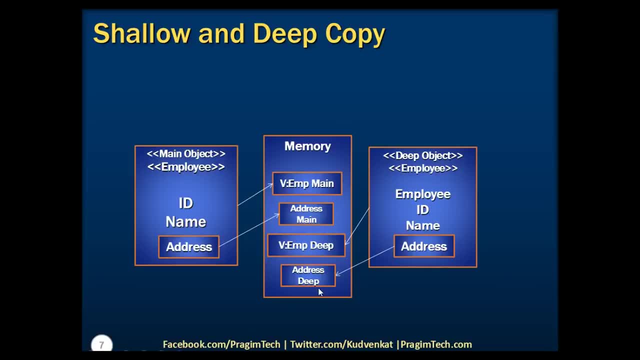 a new copy of the target objects. If you take a look at the representation diagram of deep copy post copy operation, a new location is allocated in memory for address object in the deep copy mode. We can say that deep copy copies the primary and inner object with a new instance in memory. 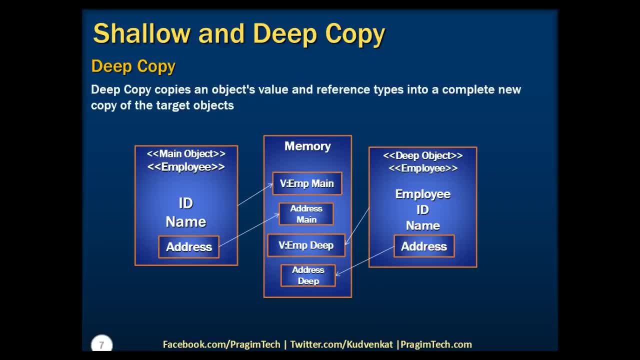 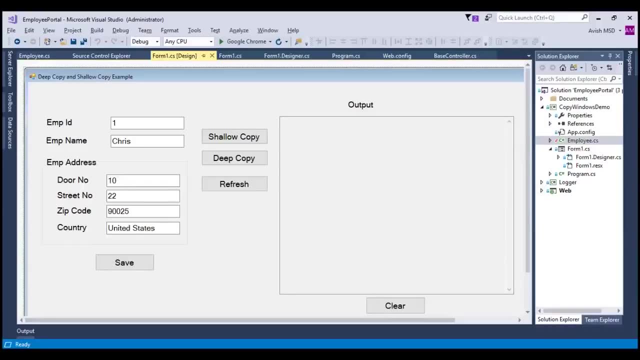 Let's now switch to visual studio and see shallow and deep copy in action with an example. In order to demo the application, I have used a simple windows form application that performs shallow and deep copy on an employee object. This application consists of text controls. 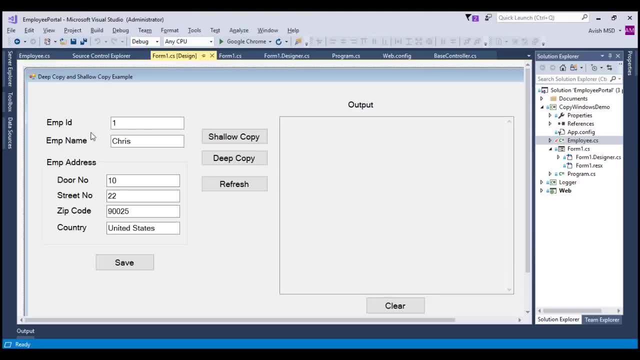 through which we can enter the employee details, such as id name and address address. address address: address address. I have also created few button controls with action methods to perform save shallow copy and deep copy on the employee details. Now let's switch to the employee class. 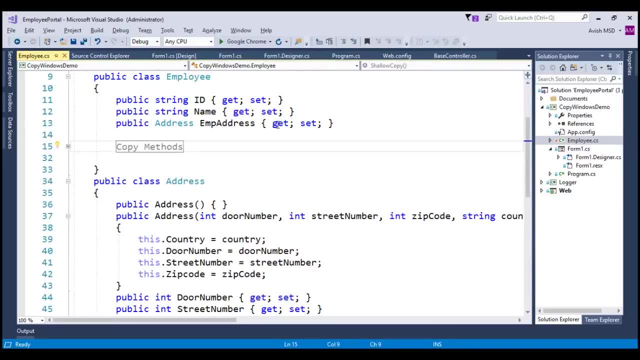 If you take a look at the employee class definition, you may notice that we have an employee class with id name and address as a default. If you take a look at the employee class definition, you may notice that we have an employee class with id name and address as the properties. 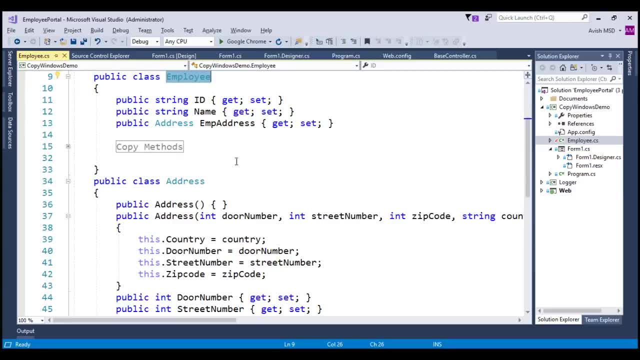 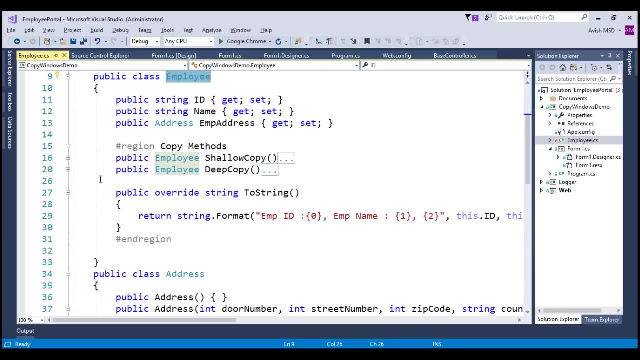 I have also created methods to perform shallow and deep copy on the employee object. Explaining the code of shallow and deep copy is out of scope of the session. The entire code is posted on the blog and we would encourage you to go through the blog for more details on the. 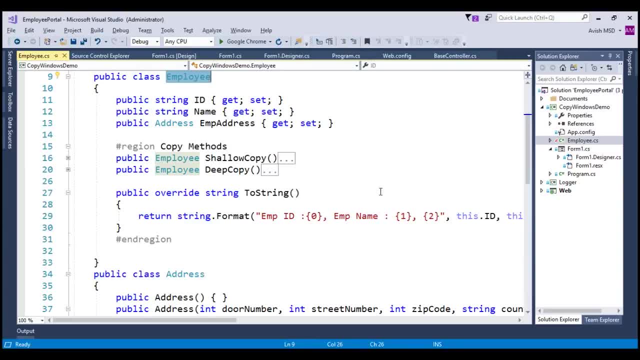 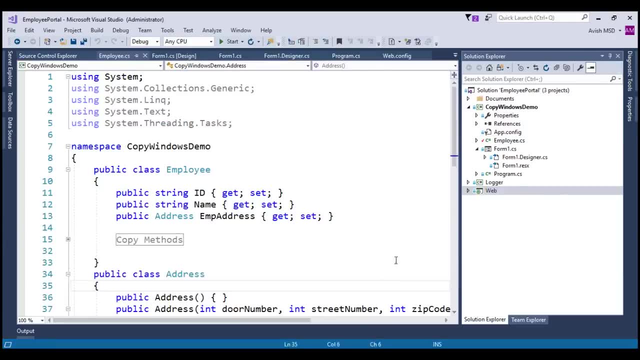 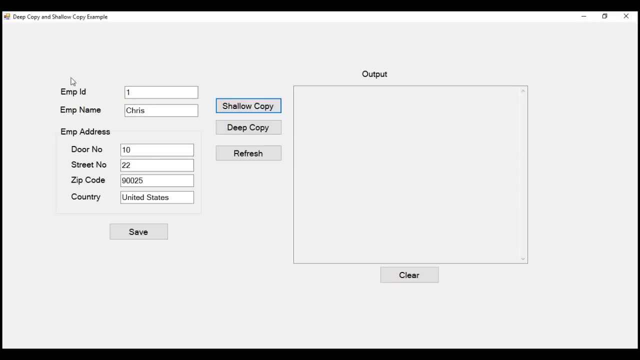 code and powerpoint presentations. let's now quickly run the application and see the differences between shallow and deep copy in action. let's run this application. you may notice that i have pre-filled the employee details. to make the things faster, let's click save and then do a shallow. 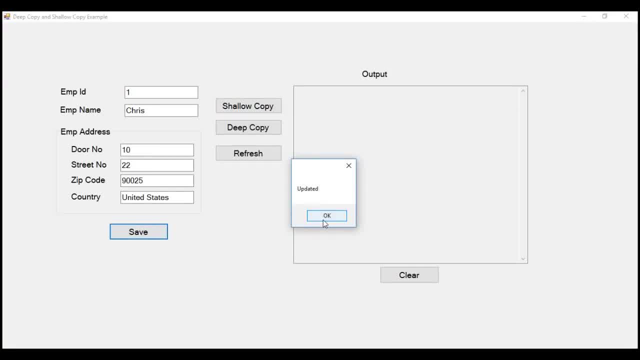 copy. look at that. the employee details are updated now. let's click on shallow copy. notice that shallow copy has copied the employee object details including name, id and address to a target employee object to prove that address in the source employee and target copied employee object are referring to the same position. let's update the. 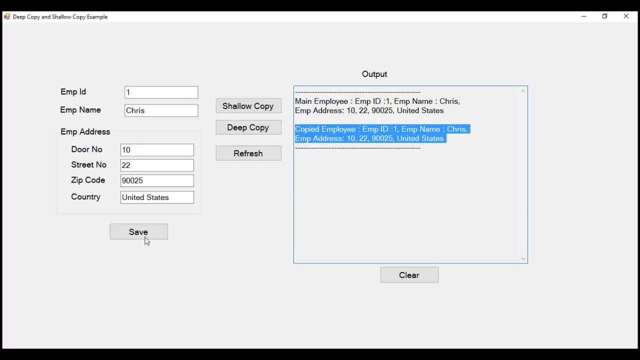 employee address and refresh the detail. let's update door number to level 11.. street number to 23 and zip code as 26. let's click on save and let's click refresh. notice that post refresh the address details are updated both in source as well as target copied employee objects. 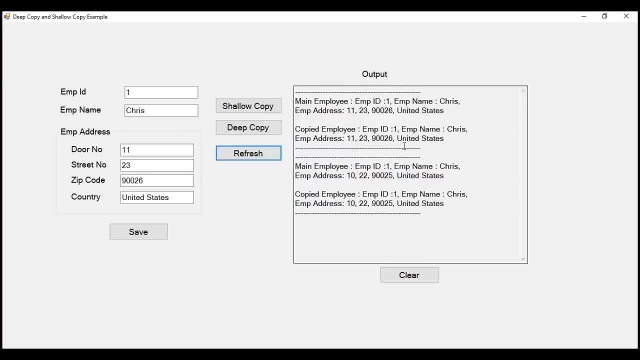 this proves that shallow copy. the inner objects are referenced to the same memory location. let's now examine the deep copy behavior. let's first clear the output and then let's do a deep copy. notice that the deep copy has copied the main employee object to a target employee object. let's now change the address details. 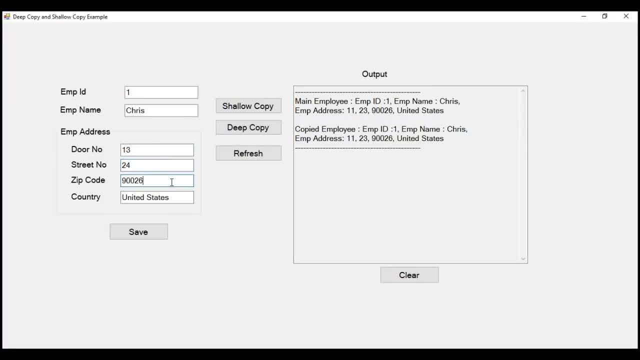 13 street, number 24, zip code 28, and let's click on save. the address details are updated. let's now click on refresh. now please notice that the address of the target employee object remain unchanged. this proves that deep copy has copied the entire employee object and created a new memory reference for. 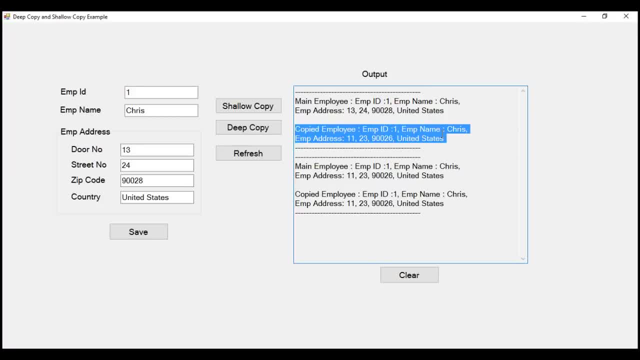 the target employee address property. i hope now you are familiar with shallow and deep copy. in the next session we will discuss the significance of shallow and deep copy in the prototype design pattern. thank you for listening and have a great day.